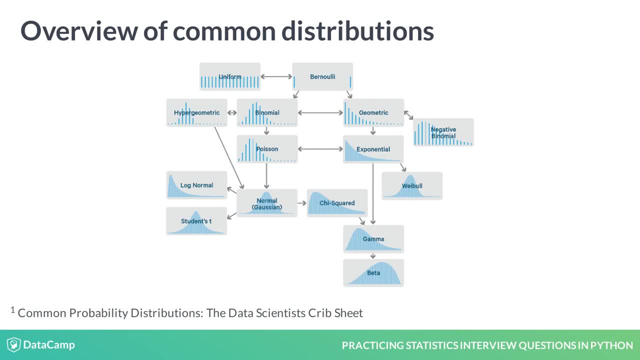 There are hundreds of distributions out there, but only a handful actually turn up in practice. In this course we'll address only the most likely to be brought up in your next interview. These include binomial Bernoulli, normal and Poisson. 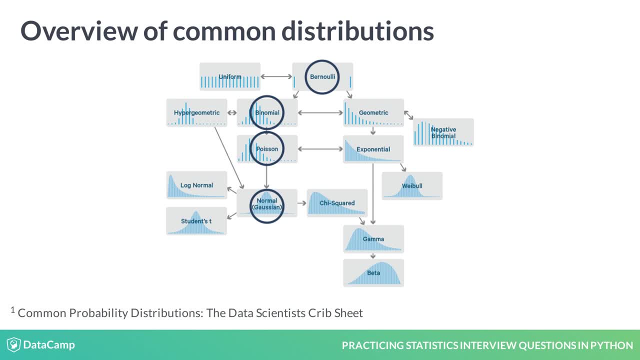 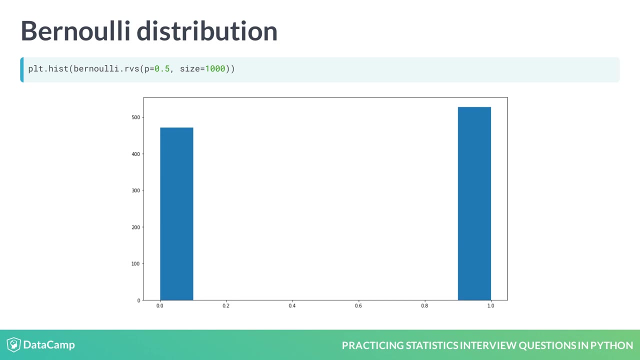 We'll use the following: Use the RVS command in SciPy to simulate all of these distributions before you visualize them using Matplotlib. Let's talk a bit more about each one. First up is Bernoulli, a discrete distribution that models the probability of two outcomes. 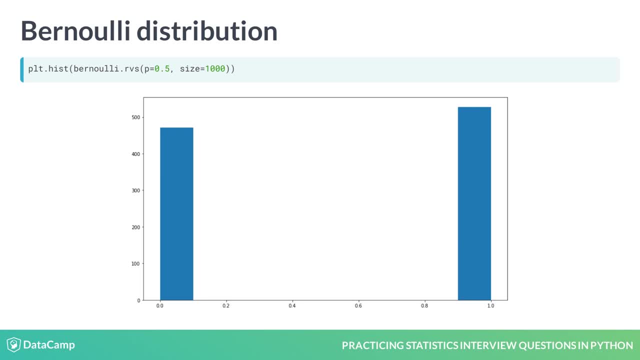 Here we see the results of a coin flip, a common Bernoulli example. Both heads and tails have the same probability of 0.5, so the values are even in this sample. Next up is the binomial distribution, which can be thought of as the sum of the outcomes. 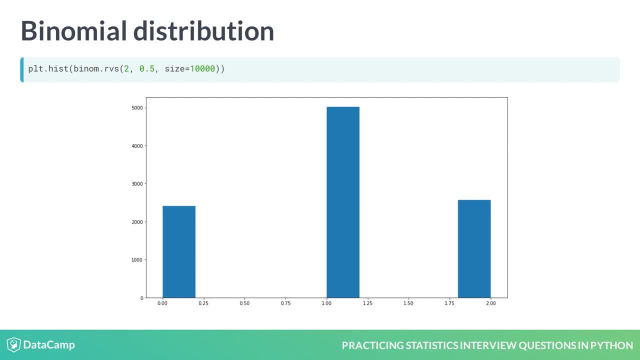 of multiple Bernoulli trials, meaning those that have an established success and failure. It's used to model the number of successful outcomes in trials where there is some consistent probability of success. These parameters are often referred to as k: the number of successes. 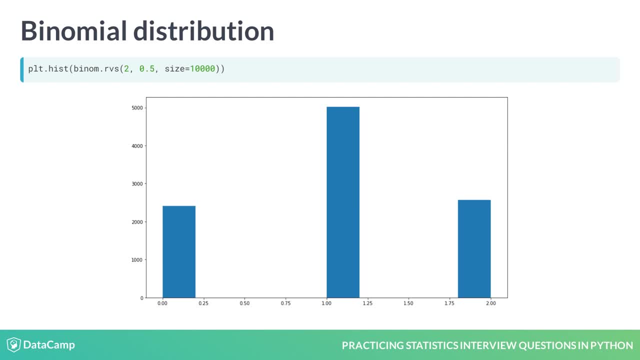 n- the number of trials and p- the probability of success. You can input these parameters into the CDF and PMF functions in Python. Here we see the results of a sample representing the number of heads in two consecutive coin flips using a fair coin, taking the form of a binomial distribution. 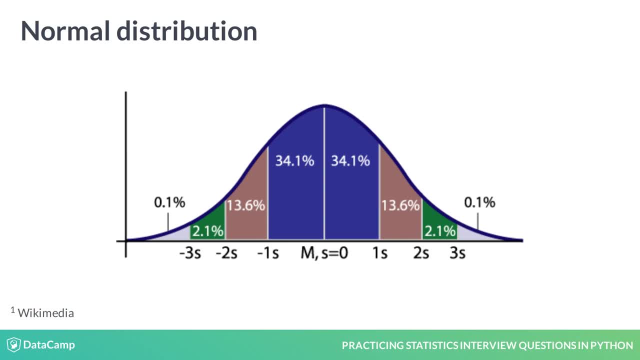 We talked a little about normal distribution when we worked through central limit theorem, but it's well worth its own slide here. The normal distribution is a bell curve shaped continuous probability distribution that is fundamental to many statistics, concepts like sampling and hypothesis testing. Here we see the normal distribution with the numbers overlaid that serve as a reminder. 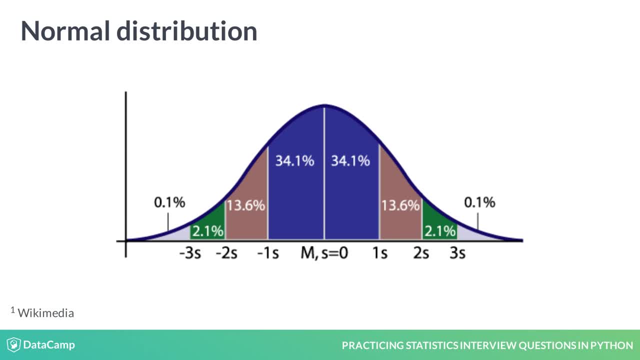 of the 68-95-99.7 rule, which states that approximately 68% of observations fall within one standard deviation of the mean, 95% of observations within two standard deviations and 99.7% within three deviations. It's good to have this memorized.